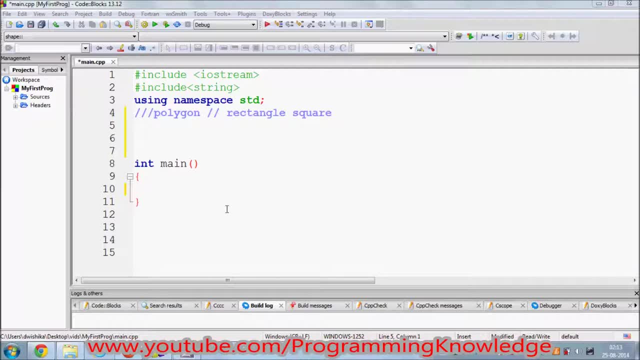 allows us to define a class in terms of another class, right? So, once again, inheritance allows us to define a class in terms of another class, which makes it easier to create and maintain our application, And this, in result, will increase the reusability of code and faster implementation. 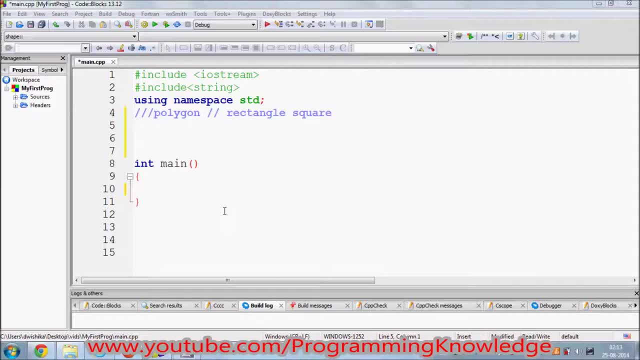 of our code. So let me give you an example. For example, you want to calculate the area of some shapes and this shape is a polygon, right? So what a polygon can be. Polygon can be a rectangle, polygon can be a square, polygon can be even triangle, right? 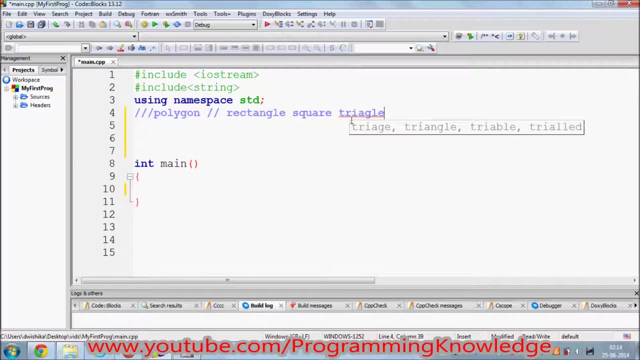 And why I'm saying this is because each of the polygon has similar property. And what is the property? Every polygon- rectangle or square or triangle- have height and width. okay, So height and width are common to each polygon, But the calculation of the area of 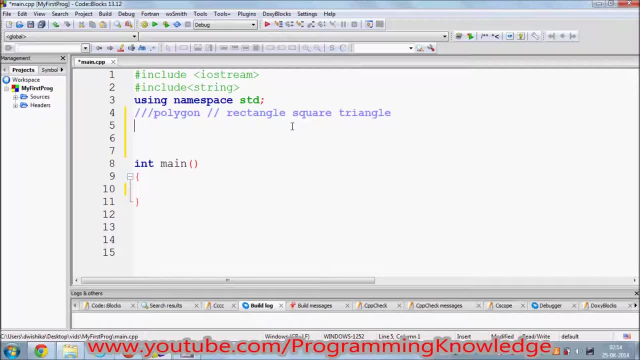 the polygon is not the same as the calculation of the area of the polygon. So the calculation of the area of the polygon is not the same as the calculation of the area of the polygon, and the area for each of the polygon is different, right? So what we can do is we can define. 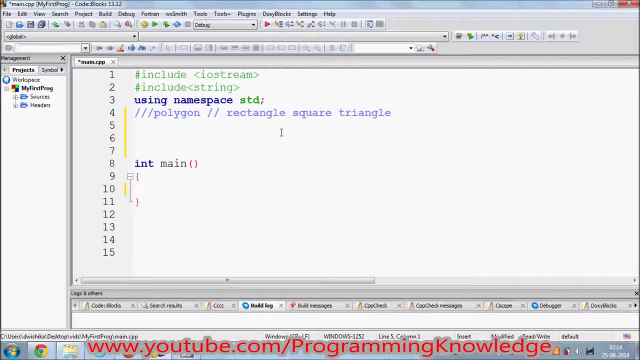 a class which have width and height that we can reuse in other class, for example, rectangle, square triangle or any other variable, So that it will reduce our code writing also and it will use the reusability of our width and height. 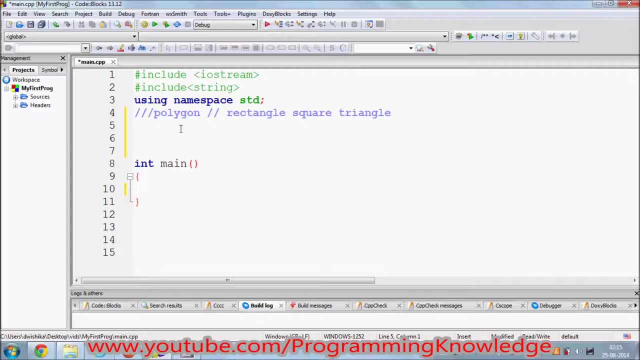 in our polygon class. so let's see how we can define inheritance classes in C++. so I have already told you, we have polygon class and in this class, for example, I named this class as shape. okay, and this class has two member variables, width and height, as I have told you. and what are these? these are protected members. now I 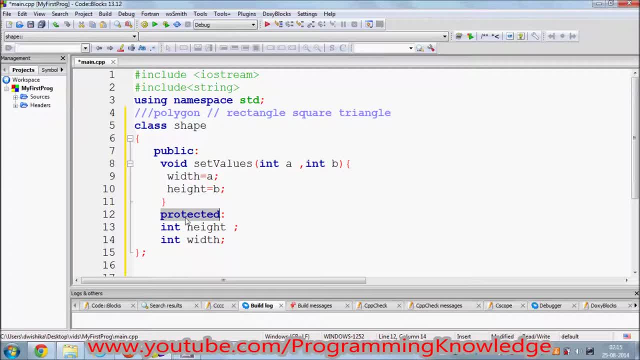 I think I haven't discussed about protected access modifier before, so this is the right time, I think. so. protected member of a class are reusable or can be used in other class, which is this class? okay, so I'm going to give you, once I complete, this example, you will be. 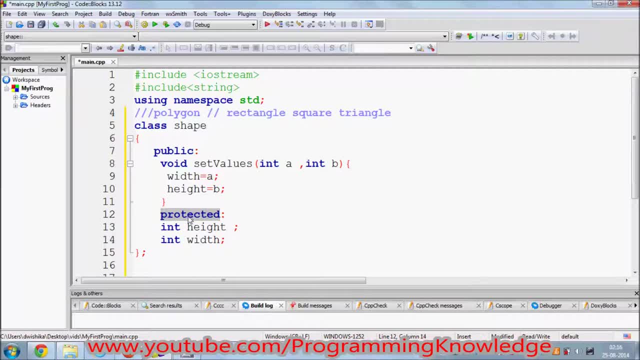 able to understand what is protected, and I will repeat this definition once again, and you already know what is public members. public members are available in other classes freely, even though they are not inheriting from the base class. so we have our class, which we call as base class. 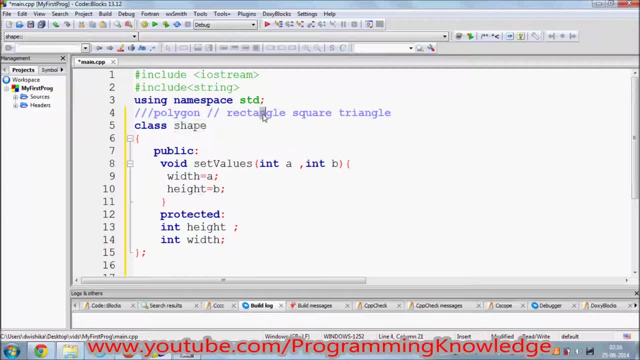 which will be a base class for rectangle, square or triangle classes, and the height and width we want to keep common to this rectangle, square or triangle class. so we have the class called shape, which has protected members, which is height and width and which has public function, function which sets, which sets these: 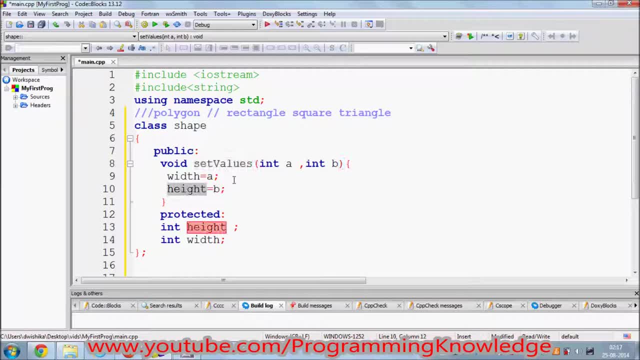 the value of width and height. okay, so this is simple function which takes two argument and whatever argument we pass it in this function, it will set the value of these two- width and height- right. so this shape is a base class. now, for example, I define our class called rectangle. 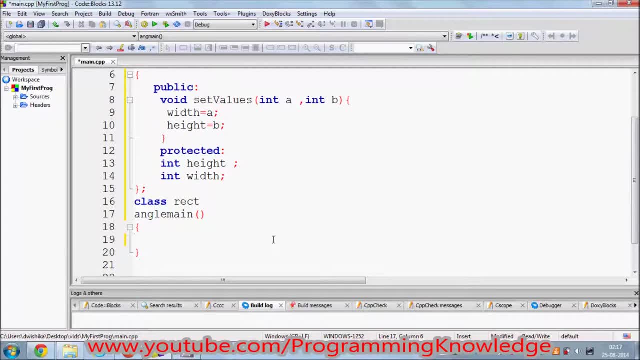 rectangle, this little bit, okay. so rectangle, and in this rectangle we want to calculate the area of the rectangle. okay, so this has public function function called void area and what it does. it it's just we are using to calculate the area of the rectangle, right? so what we are going to do, we are going to use these width and 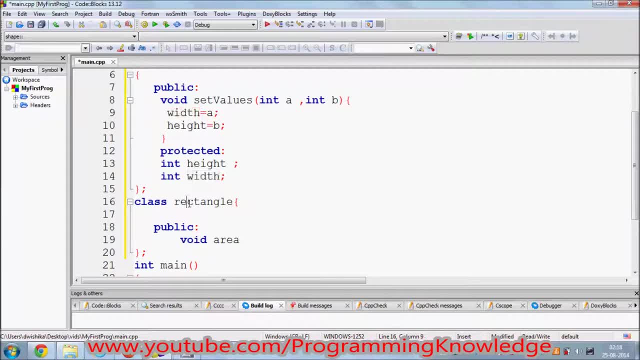 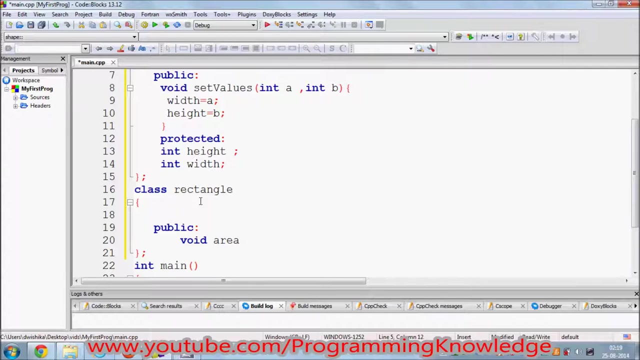 height from the shape class to our rectangle class and and how we can use it by using inheritance, and how we can inheritance- I inherit from our shape class to our rectangle class. okay, so the shape class in our case is called a base class and rectangle classes, in our case, is called 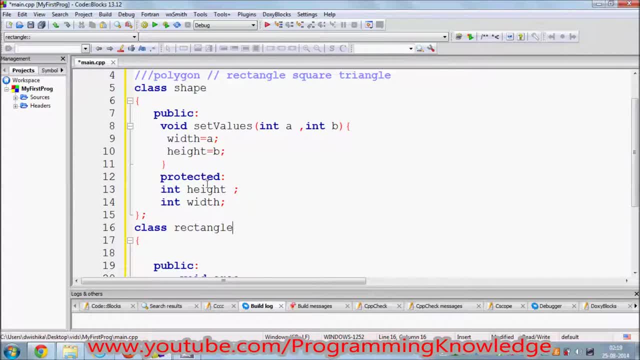 the derived class and how we can inherit from the shape class, inherit these member variables or member functions in the derived class. we just use, call a colon, this kind of colon, and then we define a access modifier which is public, public and then the name of our class from which we are deriving. okay, so this: 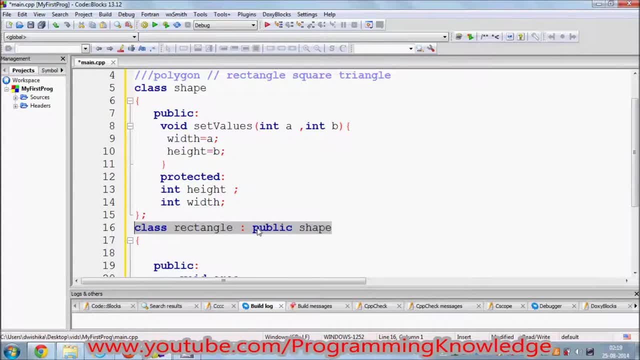 kind of declaration is called inheriting from the base class to the derived class, and rectangle, in this case, is called the derived class, and shape, in this case, is called the base class from which we are inheriting and what we are inheriting. we are inheriting height and 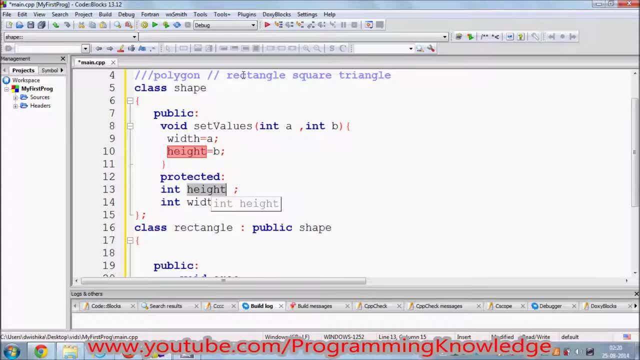 width of the polygon. okay, so we have the function, public function- and we want to calculate the area right. so what we can do, because we are inheriting from the shape class, which have height and width defined already- we can use all the public and protected members of the base class in our derived class. we can use: 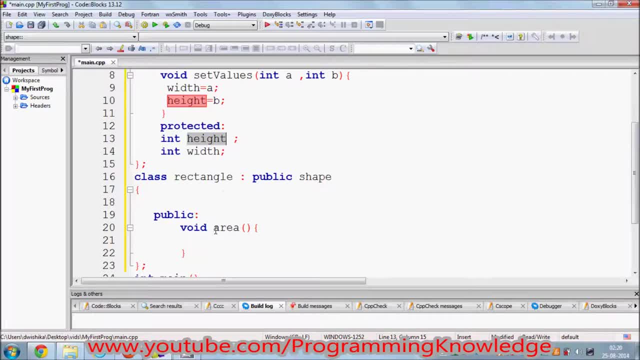 this height and width in our derived class. so what we can do: return what is the area of the rectangle height into width and because we are inheriting from shape class and these are the member variable of shape class, we can use it here also: height multiplied by width. okay, so inheritance. 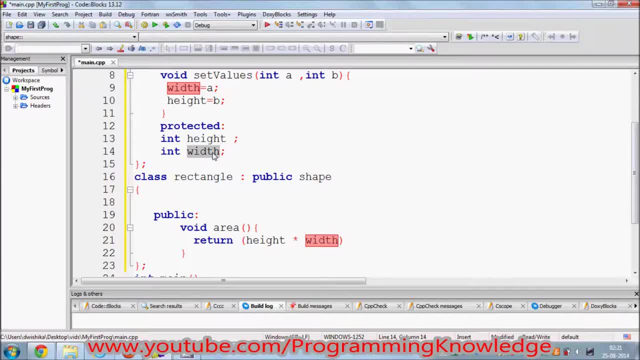 allows us to reuse the base class member variable, which are either protected or public. okay, and it will give you the area of the rectangle. right now, in order to calculate the area, let's define a other class, for example triangle, and this also will inherit from the shape class, and we also want to calculate the. 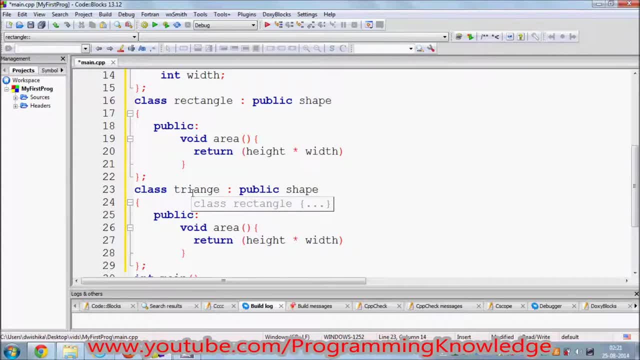 area of the triangle. so this is a class, second class, which is inheriting from the shape class, and in this class also we want to calculate the area of the rectangle triangle right. and the area of triangle is height into width divided by 2, right, if you all agree with me, I think so. area of the. 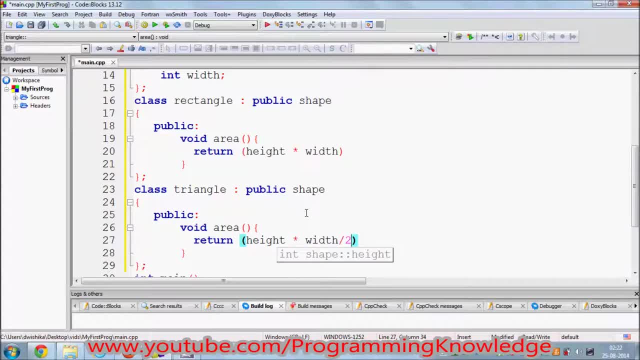 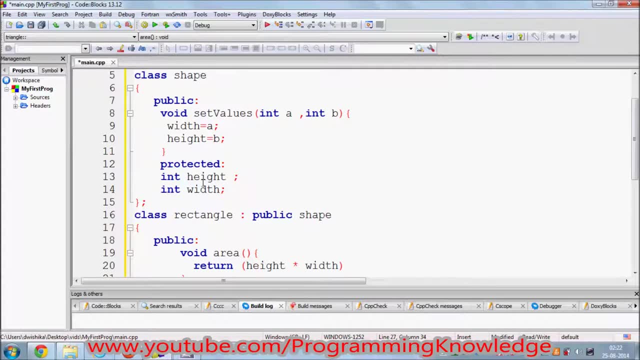 triangle is width into height, divided by 2 right. so what we are doing? we are reusing the variables from our base class in our derived classes, which are rectangle and triangle. now we can just define the object of our rectangle class. rectangle is equal to rectangle, rec. okay. and we can define the object of triangle class. 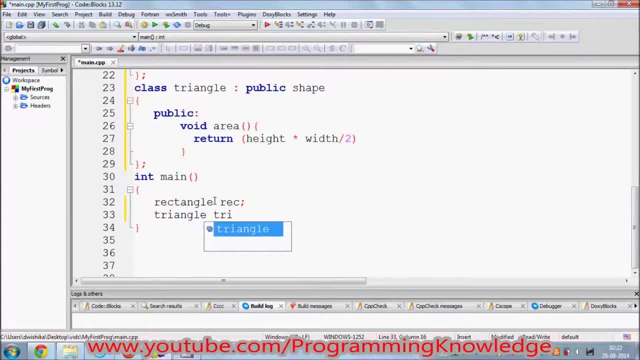 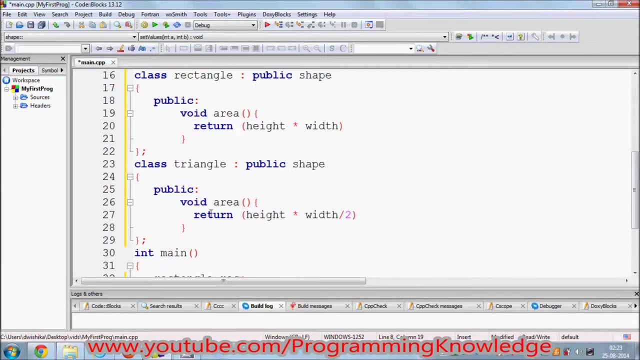 triangle, PRI, for example. and what we can do is we can reuse or we can use the function which is set value, which is there in the shape class, by using these objects called rectangle or triangle, because we are inheriting from our shape class, right. so once we write rect, which is the 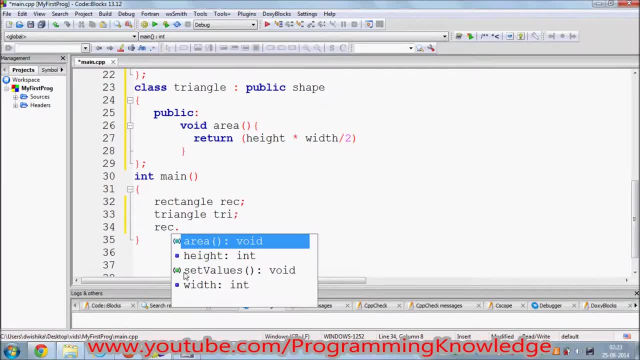 object of rectangle, class dot, and you can see here set values is available here. right, so we are going to use this and we can set. for example, we want to calculate the area width is equal to 15 and the height is equal to 10. okay, so this will give you the width and height with this. 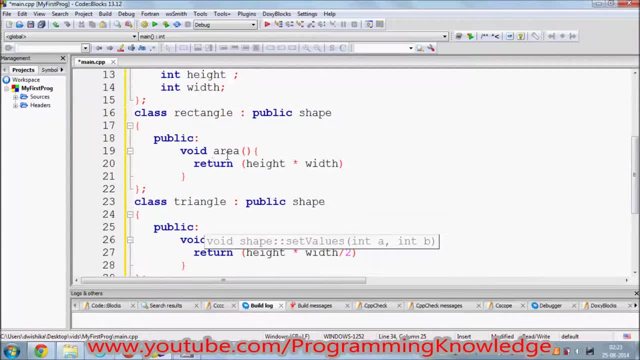 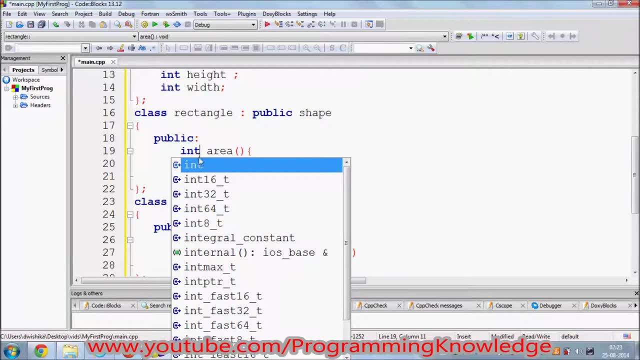 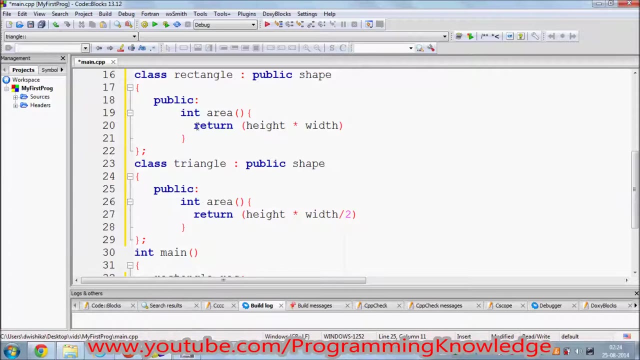 will set the width and height. and I forgot one thing: because we are returning this, we need to return int instead of void, right. you may be confused why I'm writing void here. it should be in, because we are returning integer value, right. in a similar way, I can use triangle object to calculate the. 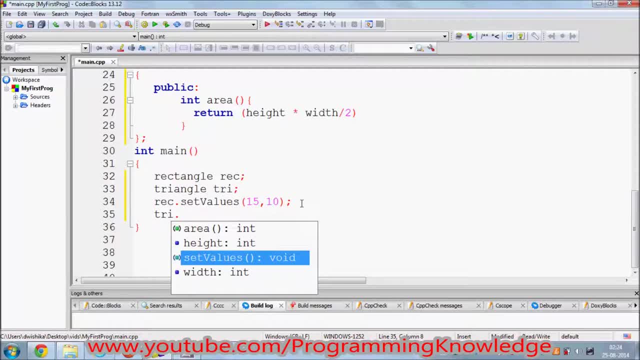 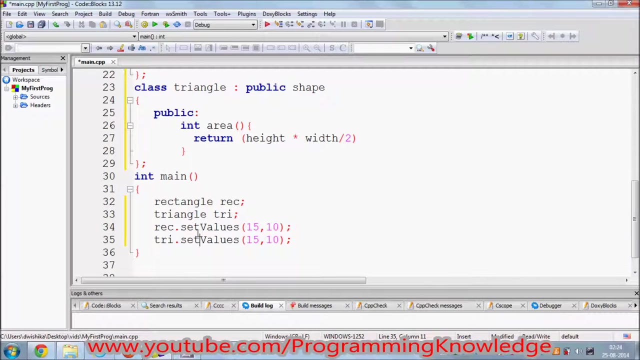 area of the triangle and the member function set value is also available here, for example, the same values I want to give in the case of this triangle to calculate the area of triangle. so this set function is there in our base class, but we can reuse this in our derived class using the object of our drive classes, right? 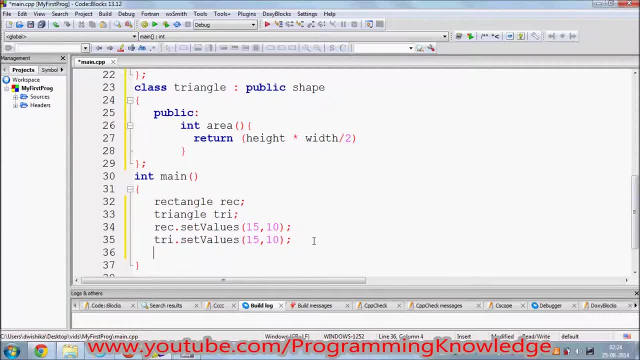 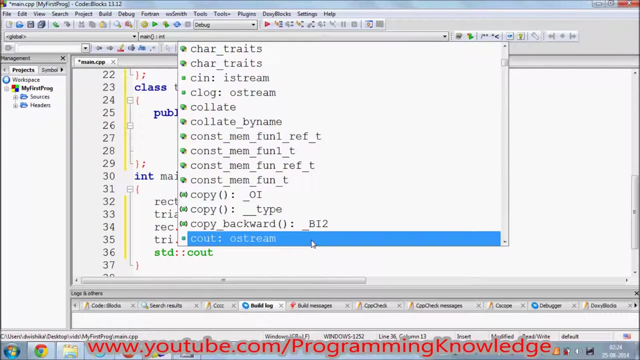 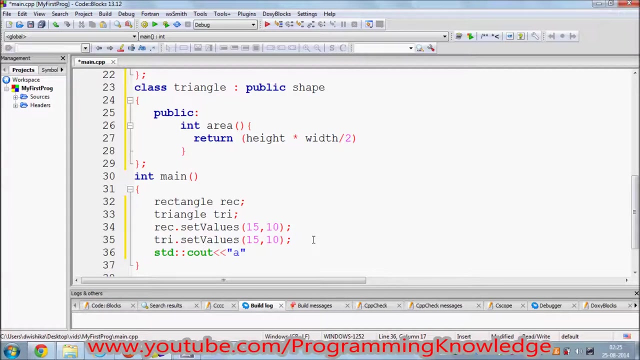 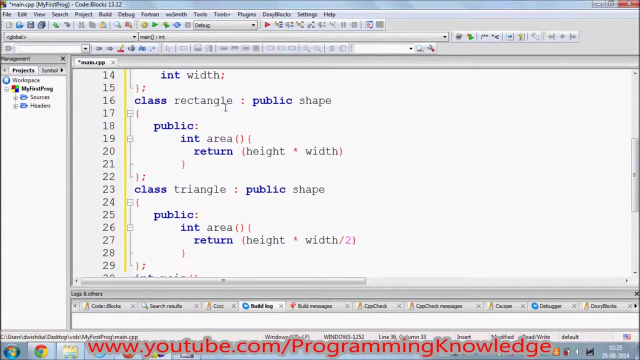 now to calculate the area, I can just write std- not here, yeah, standard, which is standard cout, and then we can just print area area rectangle is equal to, so the area of rectangle. we can find it from this rectangle function, which is a area function, right area. so we can use this. 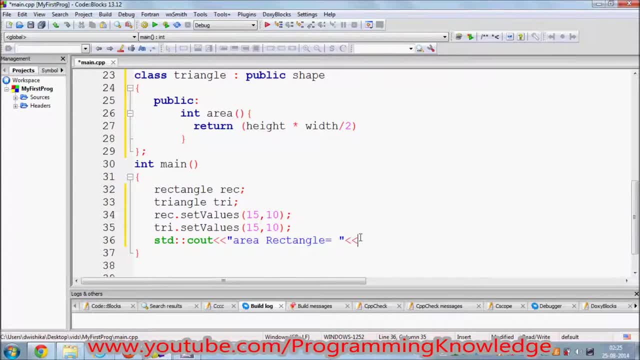 object of this rectangle class, right? so are we see dot work on the area? this will work on the if result value, which is value of area. so i need to add in on the view side so of line having this huge there in this string we can give a single line where there will be the media and a total of 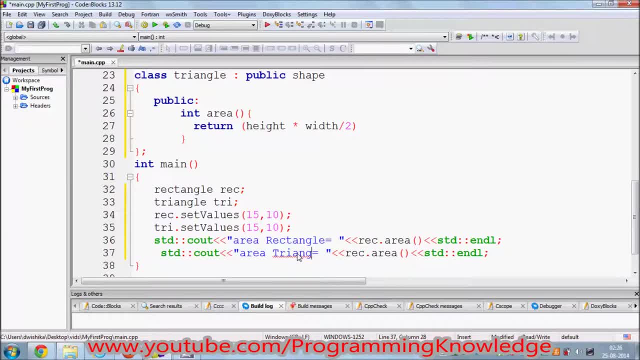 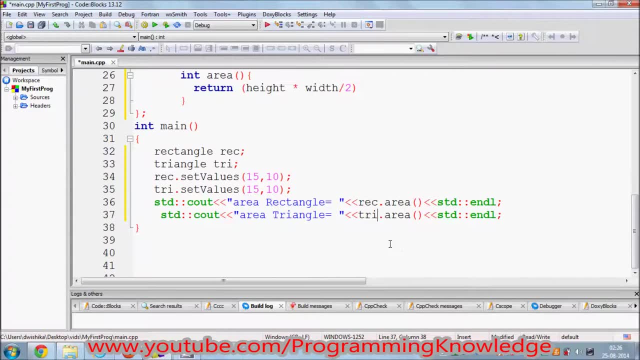 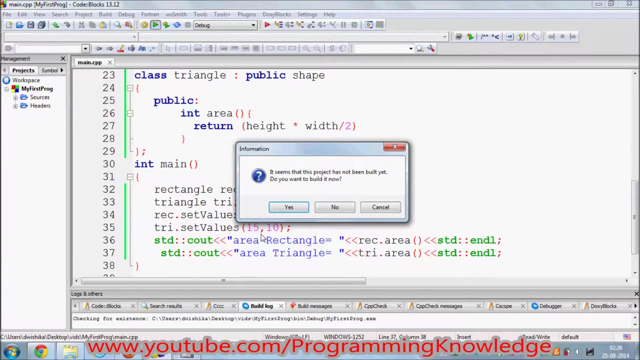 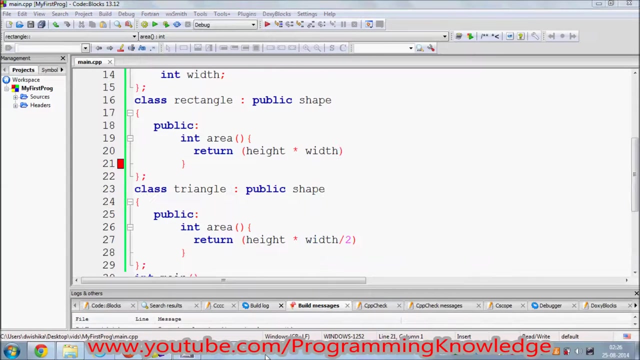 area to consist of. while this example, we get the area, but the area is enjoyed by to time. we are going to use try object, so let's try and run the program. i will just build this and, yes, we want to build it now and it gives some error. let's see what is the error. 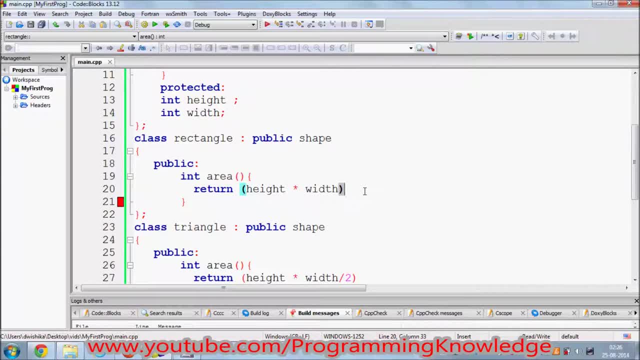 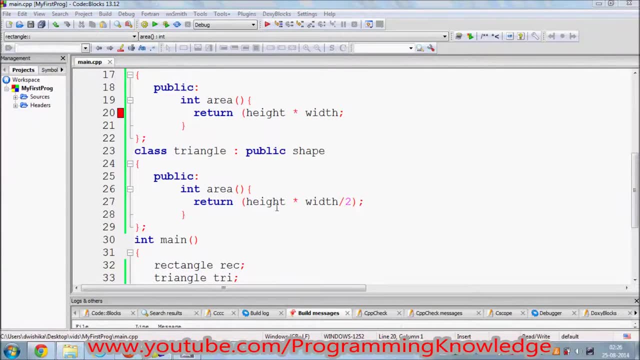 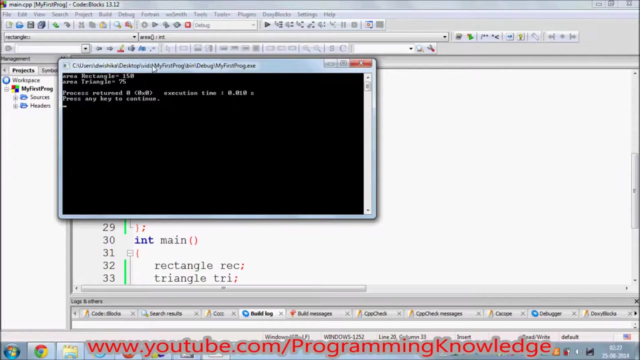 okay, so here i forgot the semicolon. here also i forgot the semicolon, and let's rebuild it once again. and still, because this has to be here and when we will build it, we can see: area rectangle is 150, which is 10, multiplied by 15, which is 150. 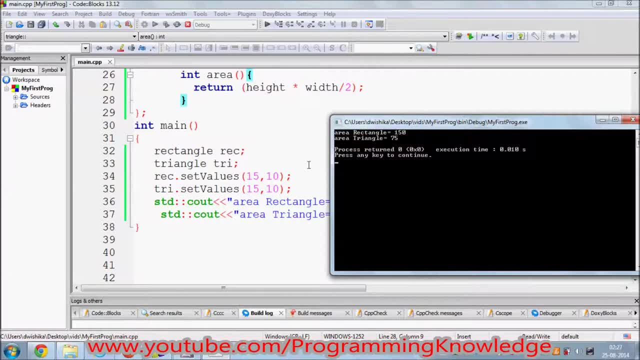 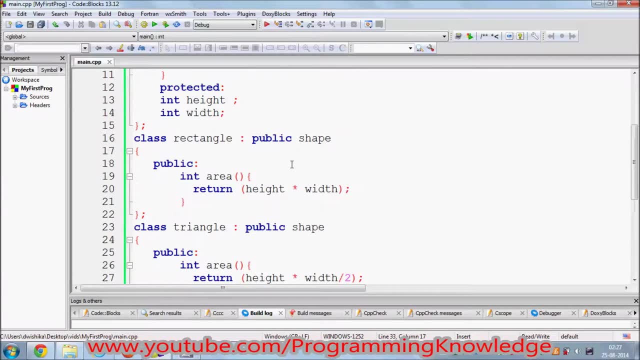 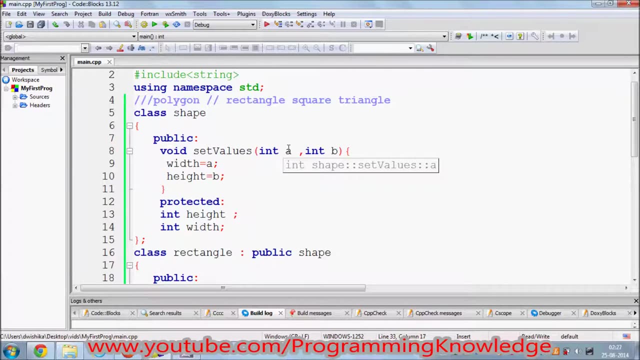 and the area of triangle is 75, which is 15, multiplied by 10, divided by 2, which is 75. okay, so this is the concept of inheritance. so, once again, what inheritance does? inheritance allows us to reuse our member functions or member variables from the base class, which is shape in our case. 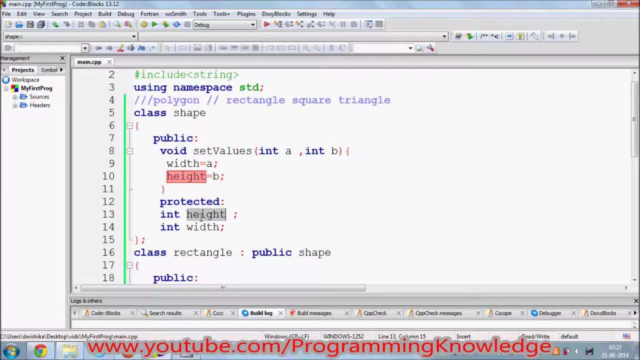 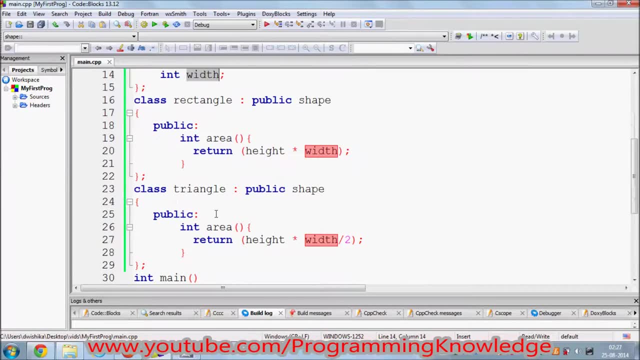 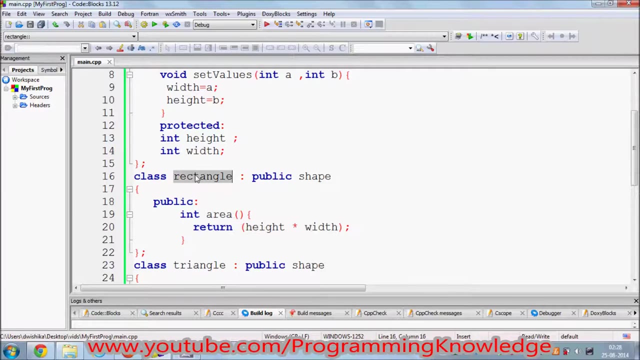 and we can inherit from shape class, because what we want, we want to reuse this height and width function in our rectangle class and triangle class, or even square class, for example, and in the derived class. so class which is inheriting from our base class is called the derived class. 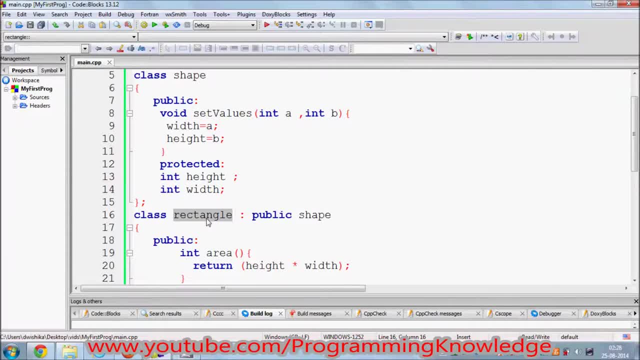 and in this week, this class has the access to all the protected members and public members of the base class. so what are protected members? protected members are the members which can be reused in the derived class. okay, so class in which we are deriving, from which we are deriving. 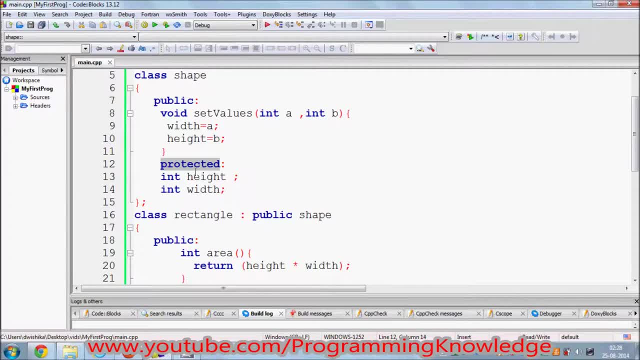 these are protected. but if it was a private member- height and width for the private member- we cannot use it in the derived class. private members are private to the class. they cannot be reused outside the class. and what are the public members? public members can be used everywhere. 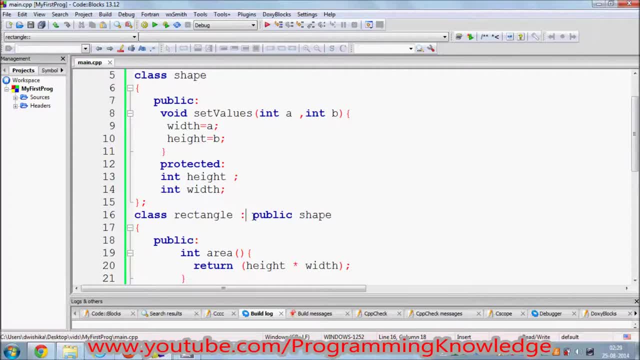 even if this rectangle class will not be derived from the shape class, even then also, we will use public members from shape class. but in order to reuse this height and width, we need to define these members- Ba謝謝 protected, because we are inheriting from this and we want to reuse this height.